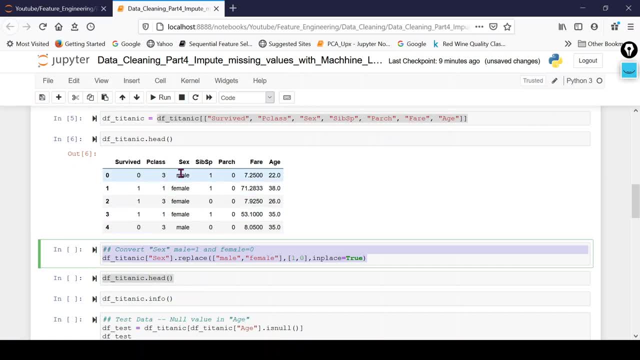 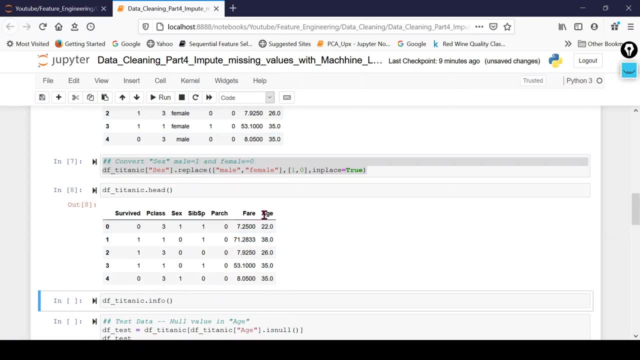 format. So what I am going to do, I am going to replace these male and female by using the 0 and 1.. Now we are going to check. yes, male and female have been replaced in numeric format. Now I am going to check the data. 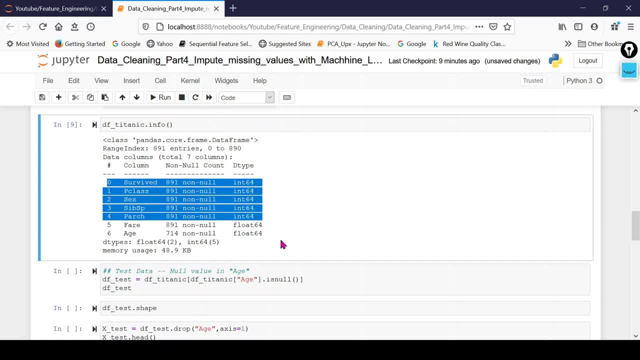 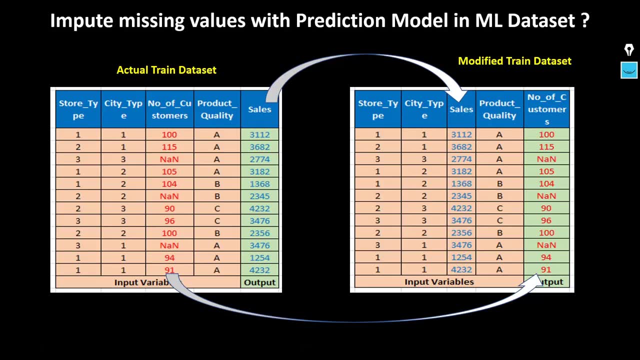 You can see all the column have in numeric format. These are float and these are all in numeric. Now what I am going to do, let me go through the slide Here. what we are going to do: we are going to use the actual training data set and we are going to modify the actual training data set into: 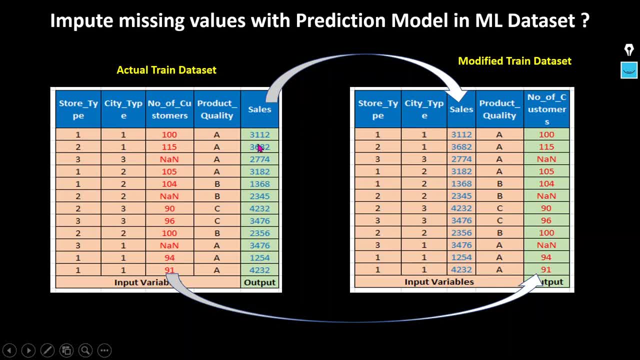 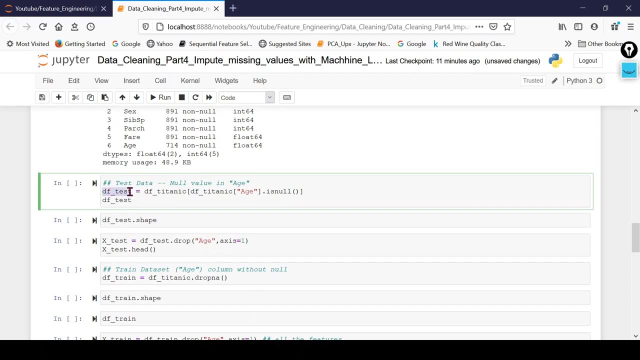 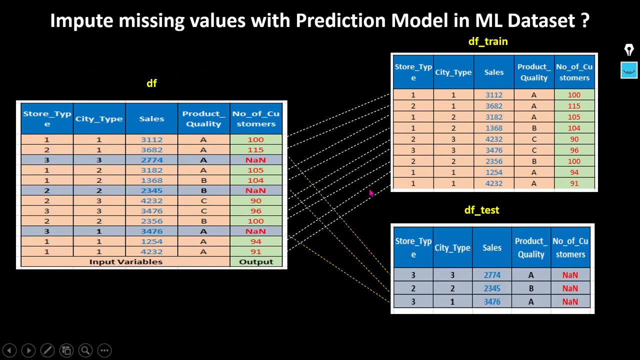 the modified training data set How we will modify. We will use the output variable as a input variable, missing value as your output variable. Same thing I am going to do here. You can see here df test How we will create the df test. You can see here df test. It means we will create df test by using: 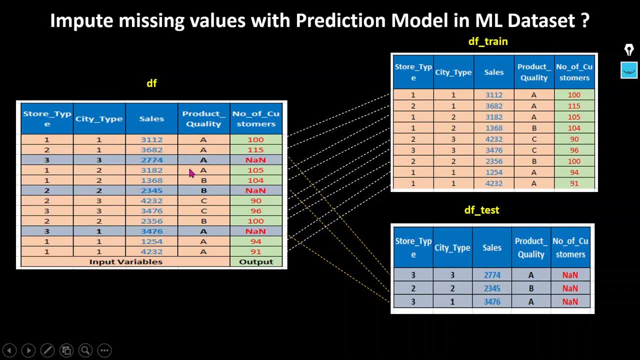 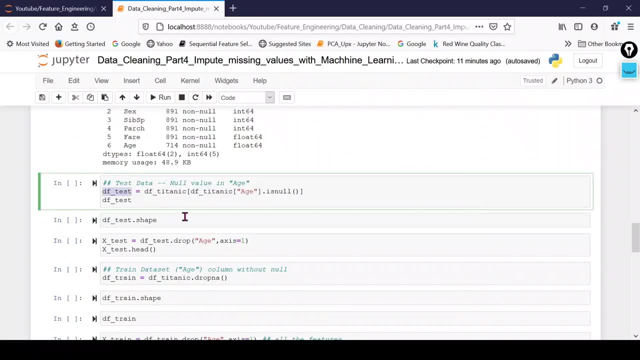 all those samples where we have the missing value in the output variables. It means this will be your age column, So all the missing value in the age column. we will use those rows And we will create a separate data frame. So let's check what I am going to do. 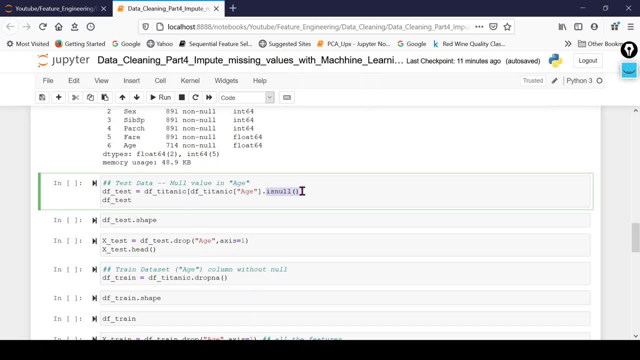 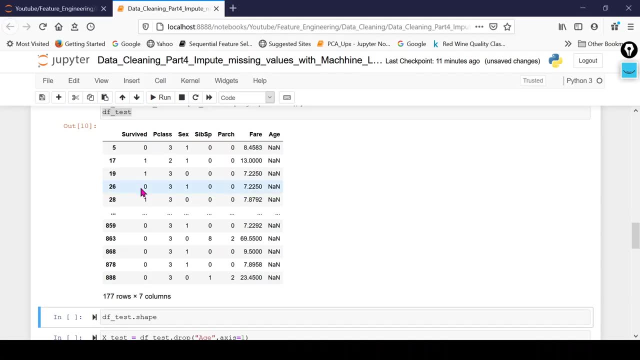 I am going to use all the missing value in the age column and creating a one data frame. You can see now this is our just like df test. This is your df test. Here we have missing value in all the rows against the age column. 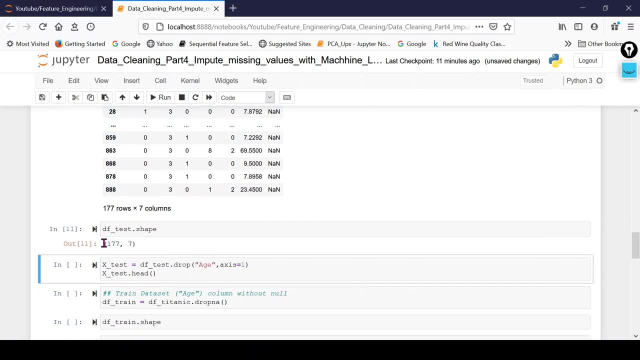 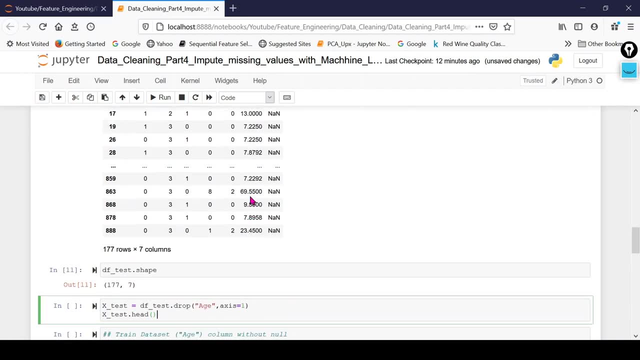 Now what I am going to check. I am going to check the shape. It means one and seventy seven rows have a missing value in the age column. now what I am going to do. I am going to drop this h column. why just check this? let this. 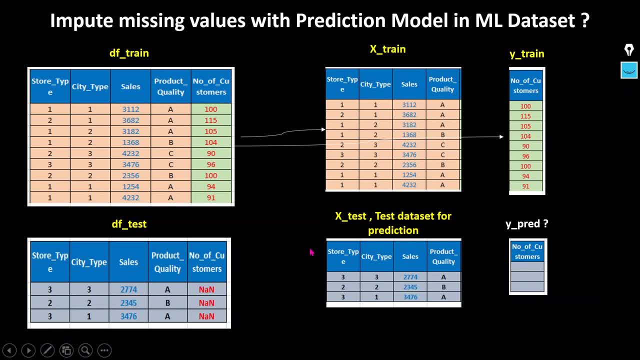 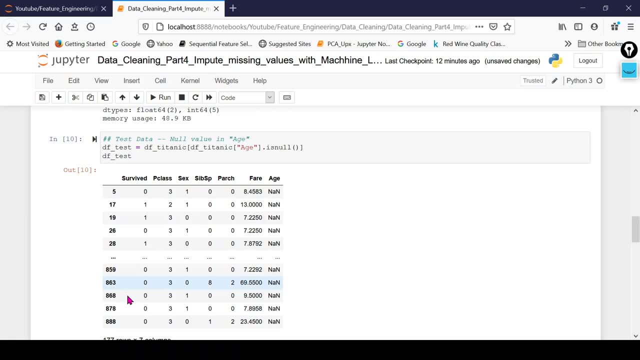 is your df test. so first we have to separate the x test and y test. this y test will be your biprad. it means we would need x test. so that's why I am going to separate the input variable and the output variable. this is your input variable till from survive to fair this. 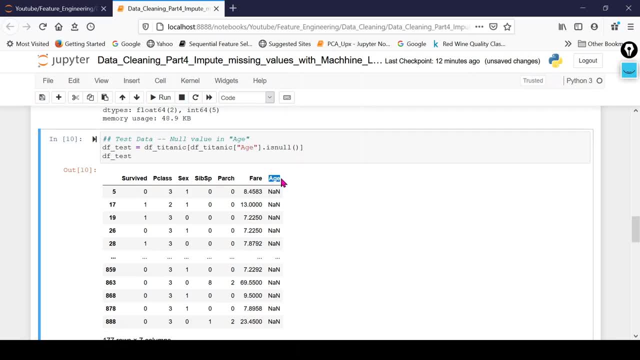 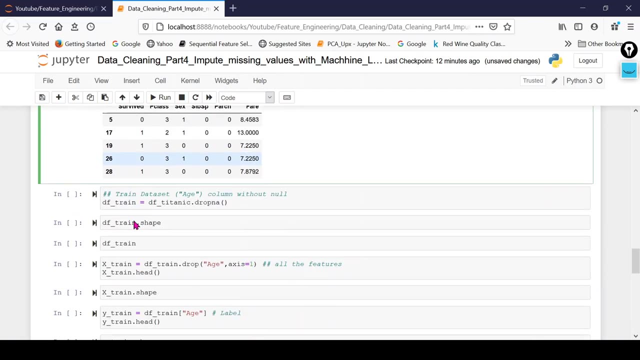 is your input variable and this is your output variable which will be work as your biprad. so how we will do that, I am going to drop the h column. h column. once we will drop the h column, we will get the x test. this is your x test. now, what I am going to do, you can see. 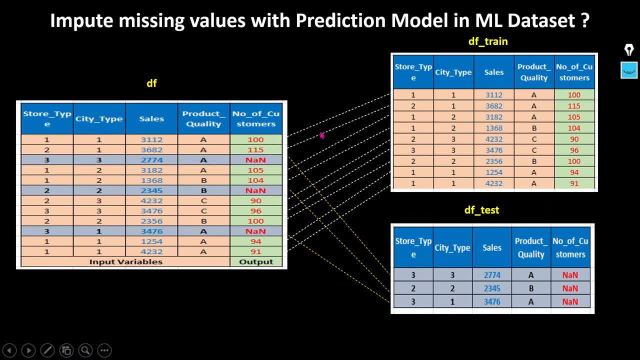 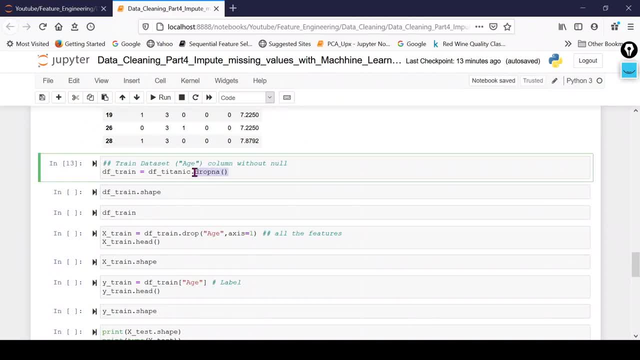 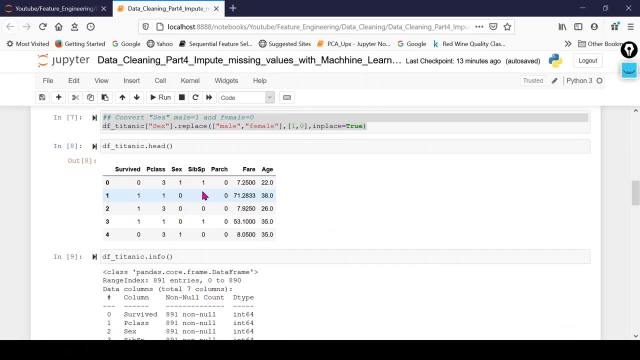 if we will drop all these rows, nan rows, then we will get this df10. so same thing I am gonna do here, same thing I am gonna do here: I am going to remove all the na columns in the existing df train. it means this data frame. 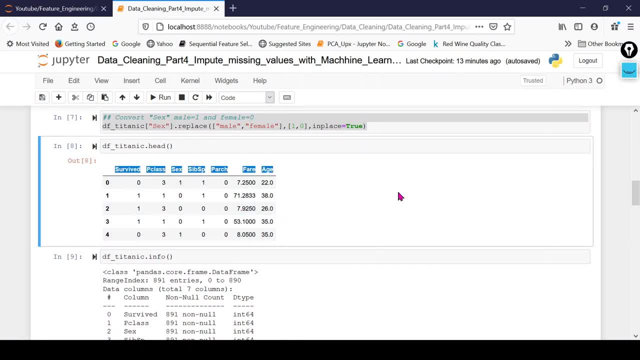 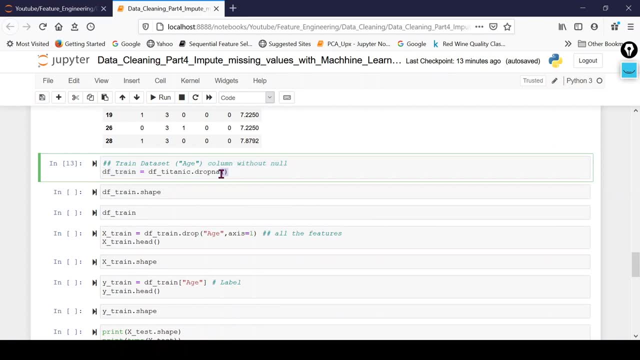 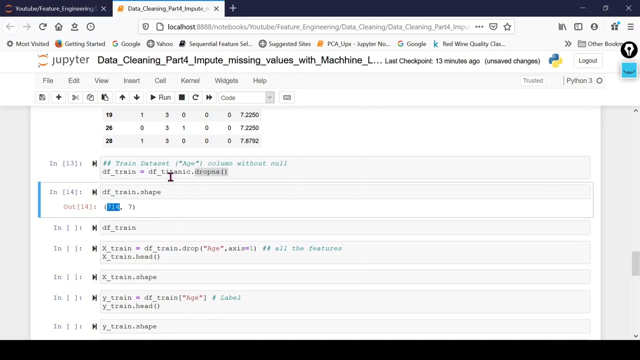 df titanic. I am going to remove all the 9 values so you can see df titanic data frame. I am going to remove all the na values so now we can see 714. it means remaining column we got, If you will add 714. 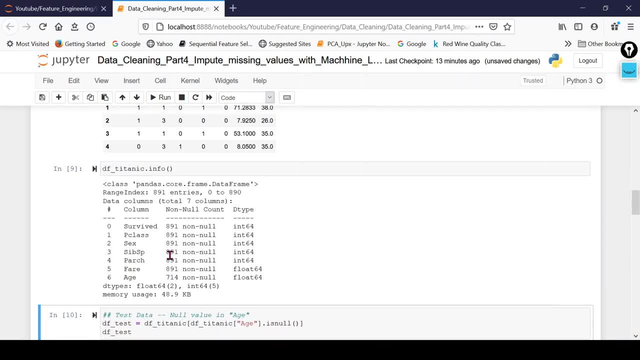 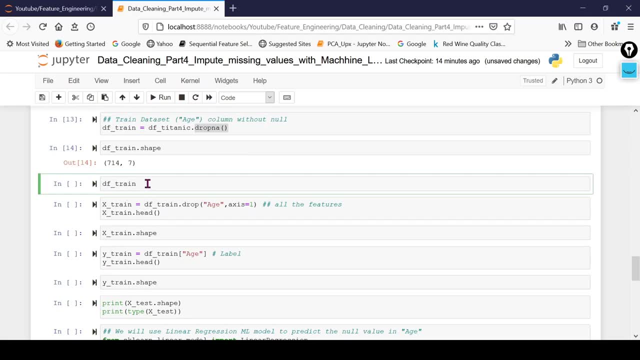 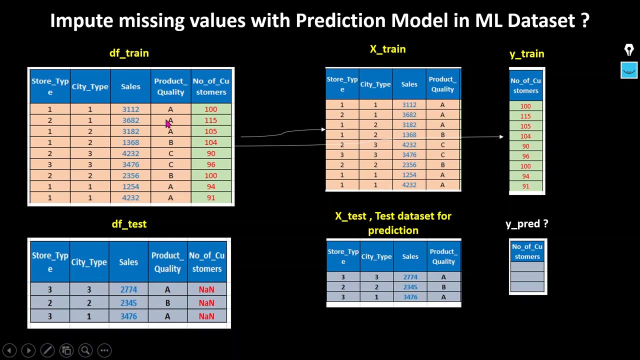 714 and 177, you will get the 891. so now we have the df train and df test, df train. we have now this: what we will do now, same thing which we did for df test, now we will do for the df train. it means separate x train and by train. x train is your input, variable by train. 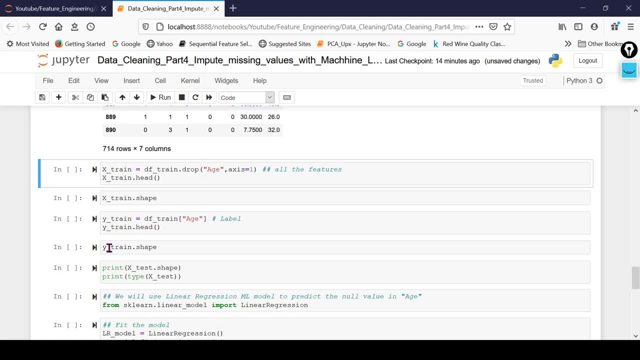 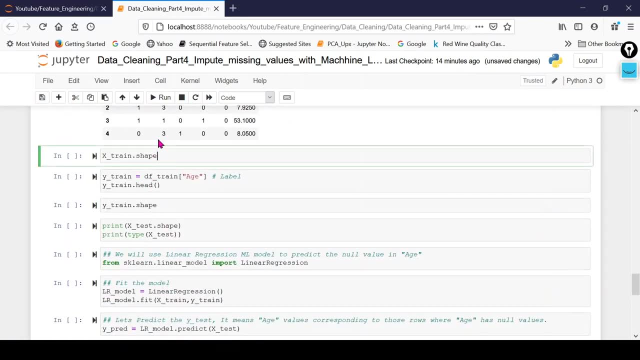 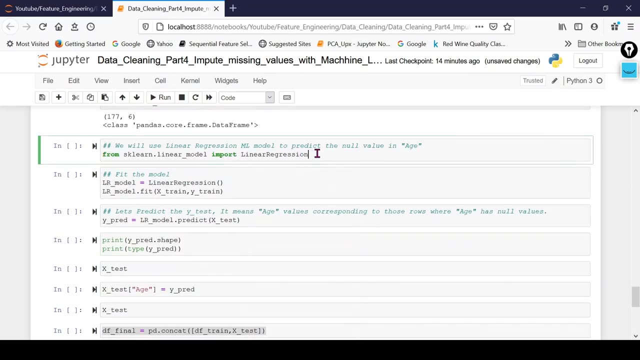 is your output variable. in our case, by train will be your h column. you can see here, x train is your input variable and this is your shape. what I am going to do by train is your h column. you can see, this is your h column. now we are going to train. 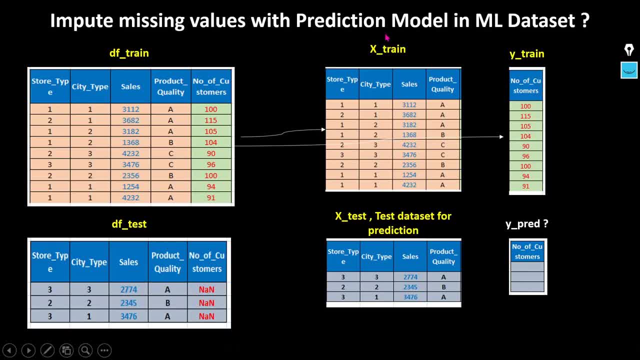 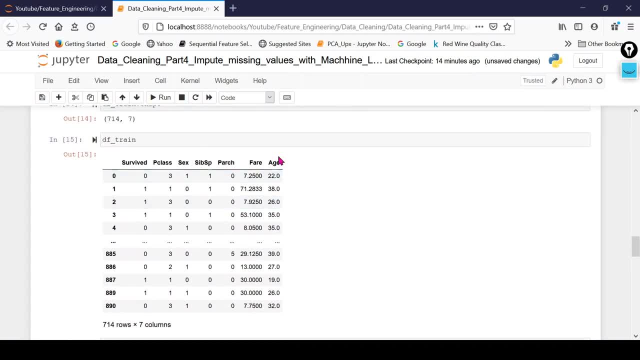 our machine learning model. we will train our machine learning model with the help of x train and by train. here our h column is your. you can see, here h column is your numeric so and it is in continuous nature, so we will use the linear column. 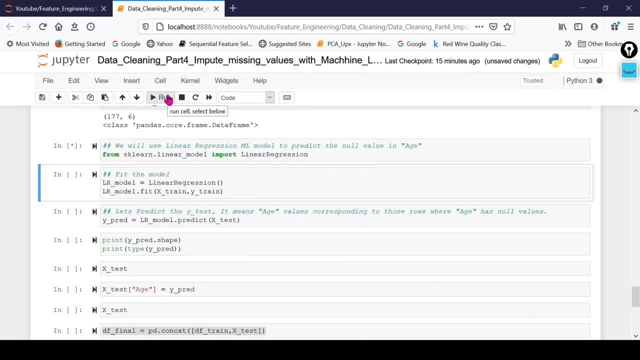 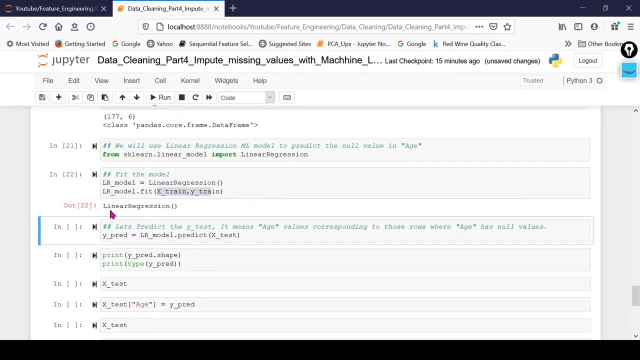 so we will use the linear column, so we will use the linear regression model. so I am going to import the linear regression library here first, then I am going to fit our x train, and by train. now our model has been trained. now, what we will do, we will predict this bipred, this bipred, with the help of this, 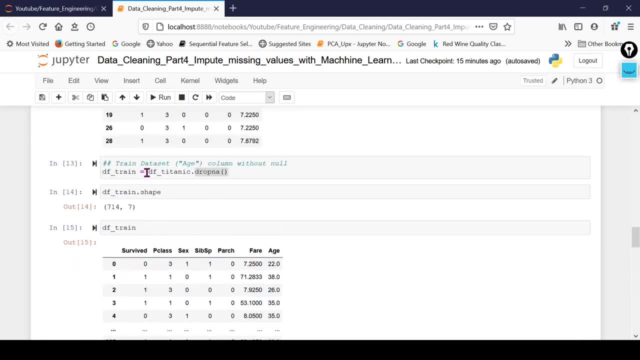 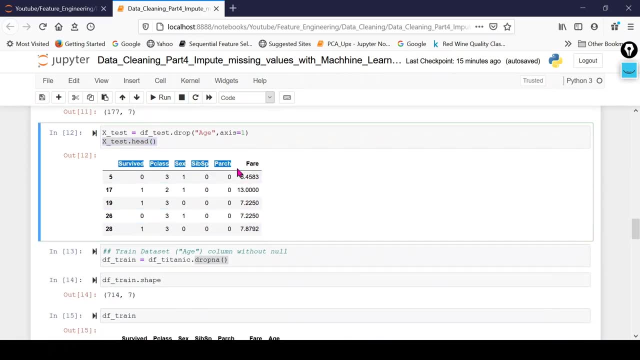 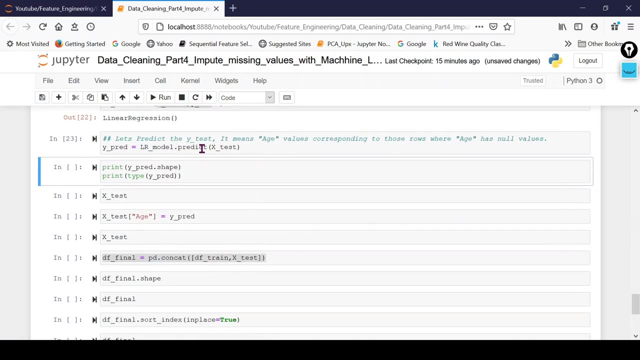 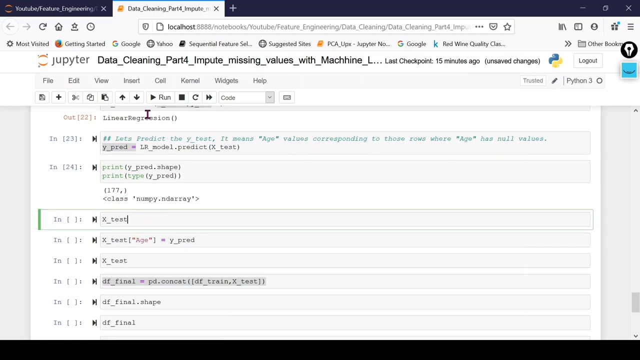 x test value. in our case, x test is your, after removing the h column, what we got here, this x test, these data we are gonna feed in this machine learning model. we are gonna feed here. now. we got the bipred here. let's check the bipred. we got 177 output. this is your x test. 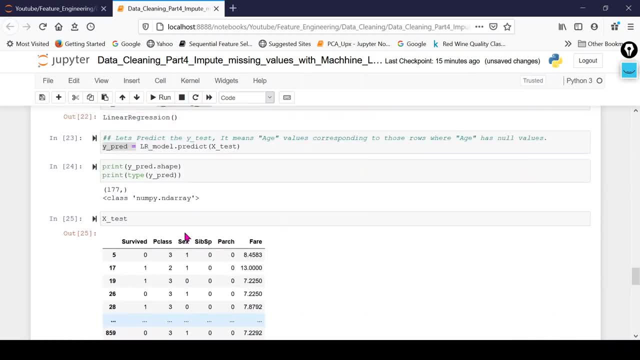 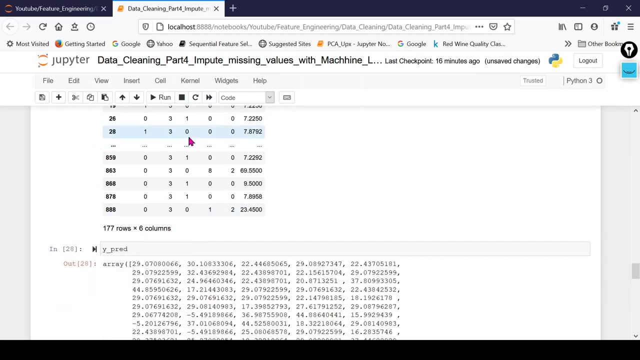 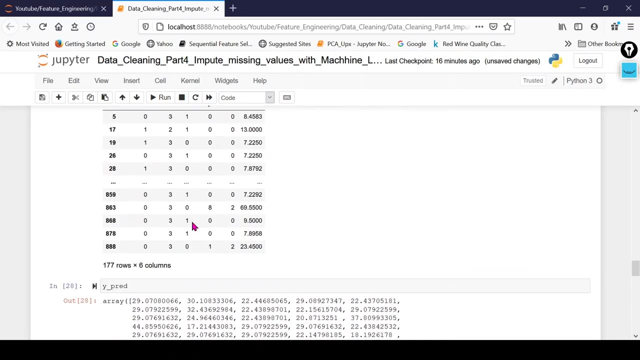 and now this is your. so what we did here- if you see, this is your x test and if I will use this bipred here, you can see this is your bipred. What I am going to do, I am going to add a one column age in this data frame- X test- and 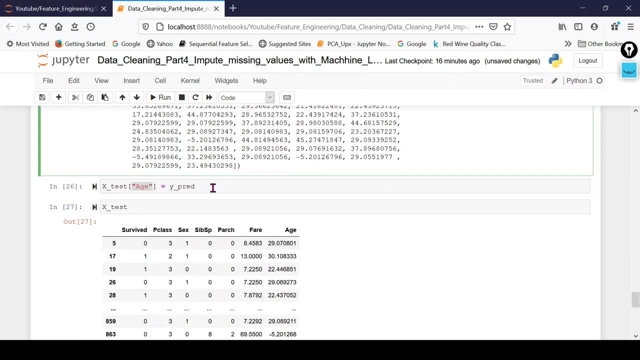 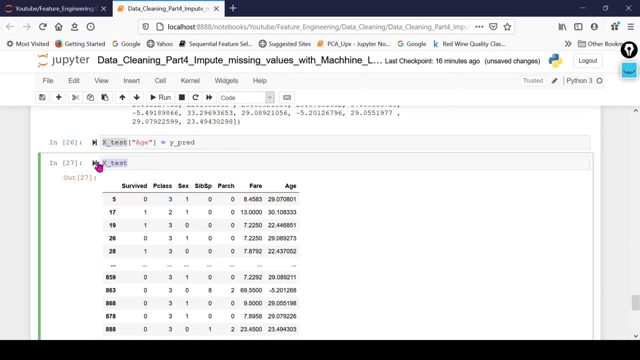 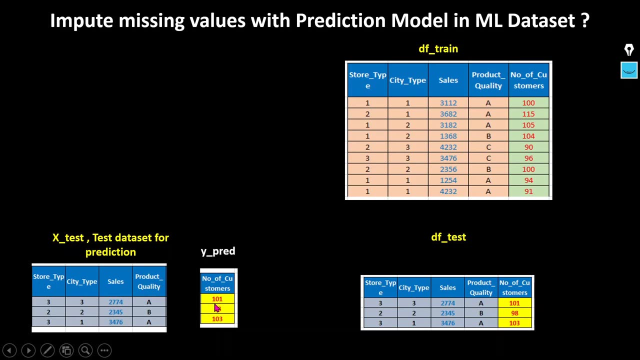 going to import all these bifred value in this age column. So after that we got this age column in this X test data frame. So this X test data frame will be your, like this data frame df test. after once we will get the predict, then we will create a one new column, age like your here. number of the. 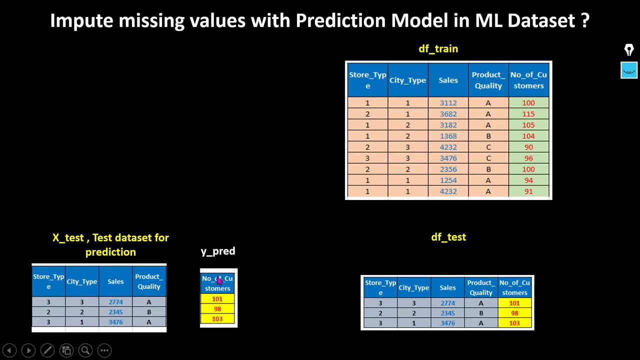 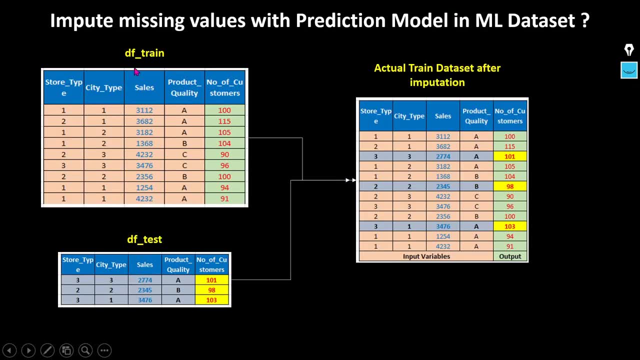 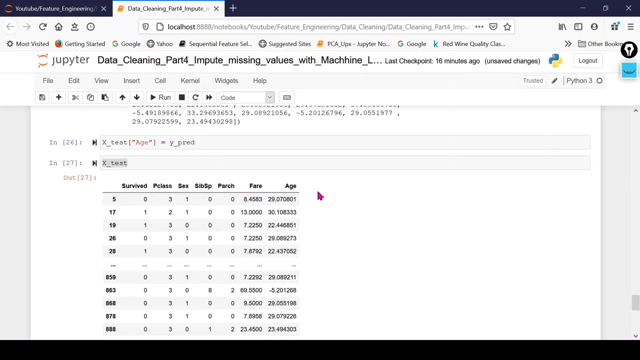 customer and will import all the output value in that particular column. Same thing I am gonna do here. So now we will. so now what we will do: we will combine df train and df test. here we are going to combine concatenation of df train and X test. df train is your actual, this one like 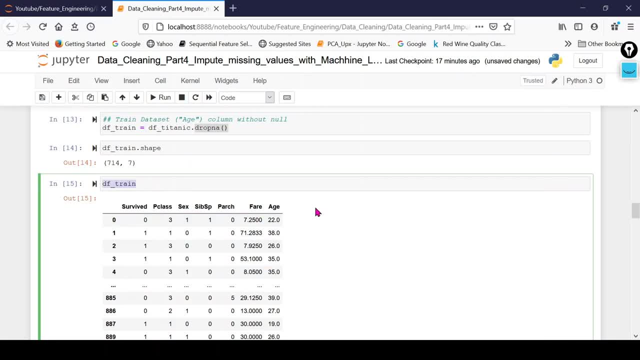 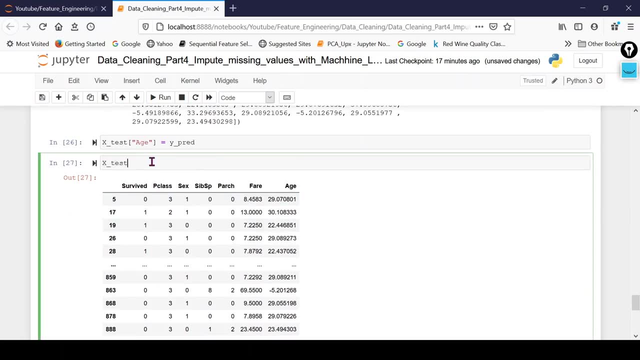 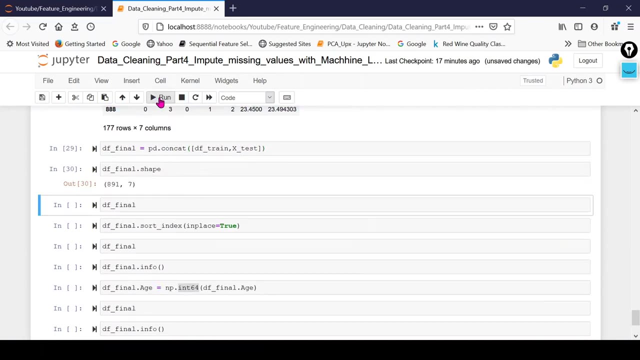 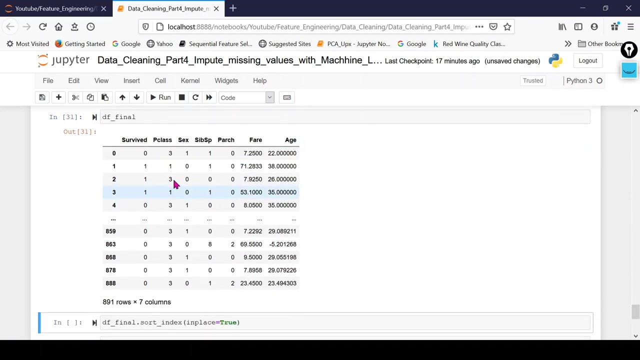 your df train, this one, this data frame, and your, after adding the age column, it means this data frame. so we are going to combine both data frame by using the concatenation. Now this is your final output. you can see our count is same: 891. so this is your final. 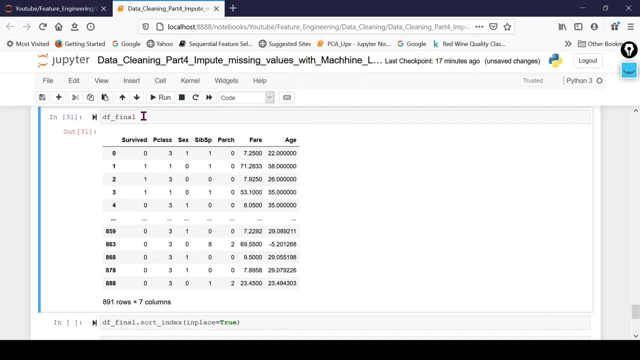 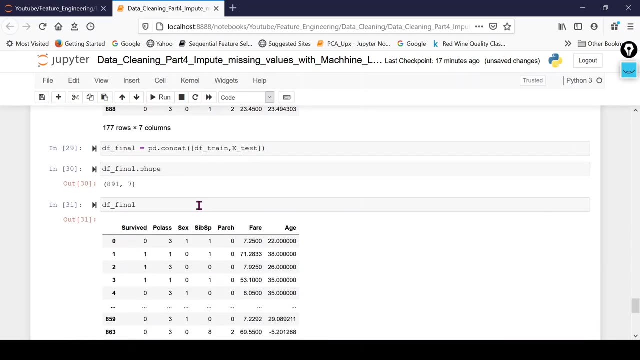 this is your final data frame, which we will use to train our machine learning model for our business purpose. Here we have removed all the missing value in the age column. here you are seeing that we are getting 000. so why what we can do? we can: first we will sort the index. why we will?